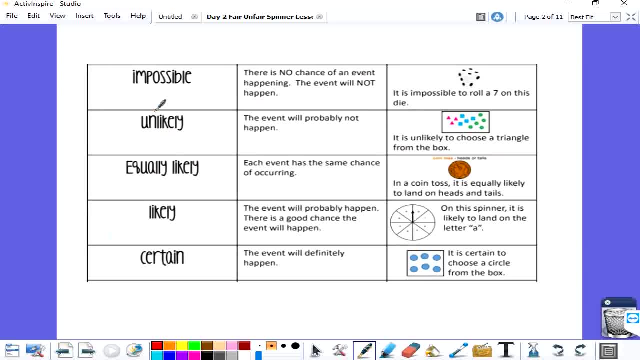 That we learned from yesterday. The first one is impossible And that just means that there is no chance of an event happening. And if you look at this die, a regular die has six sides labeled one through six. There is no number seven on the die. 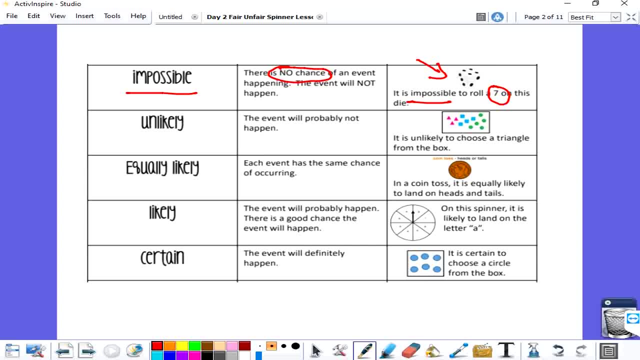 So it's impossible to roll a seven. Unlikely means that it will probably not happen. Little chance of happening. So if you look at this rectangle Right here There, it is unlikely that we're going to pick a triangle because there's more of the other shapes than any than the triangle. 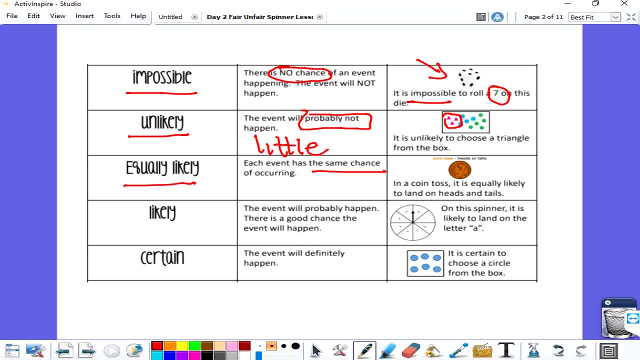 Equally likely means that each event has the same chance of occurring And I know in a coin toss it is equally likely to land on heads and tails because there is one side of each. Likely means that it will probably happen And there's a good chance it will happen on this spinner. 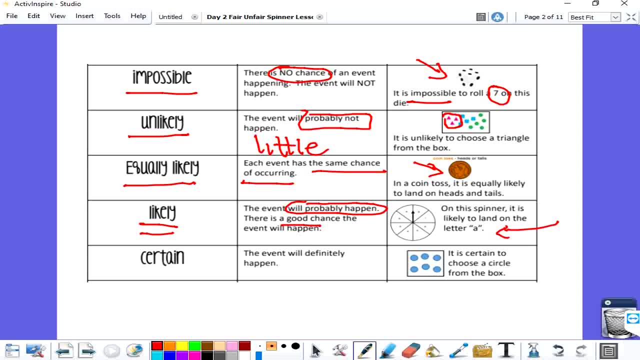 It is likely to land on the letter A, because there's more A's on that spinner than any other letter, And certain Definitely happen. I am 100% sure. If you look at this rectangle, I am certain, or 100% sure, that I will choose a circle from this box, because that's all there is in that box. 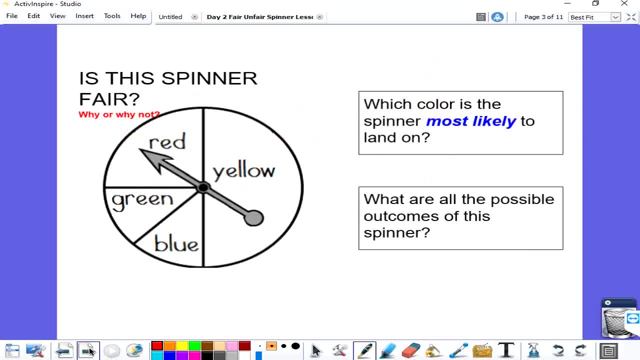 So, to begin, let's talk about fair and unfair. Is this spinner Fair? Why, or why not? Well, I'm looking at that spinner and I'm thinking that that spinner is not fair because, even though I see four colors, the pieces and the sizes of the colors are not the same. 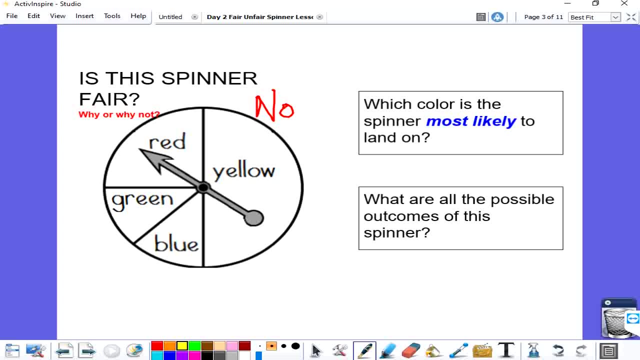 So they are not equal, So it is not fair. So let's take a look: Which color is the spinner most likely to land on? Well, if I Look at the spinner closely, I know that yellow has the biggest space on that spinner, so it is most likely to land on yellow. 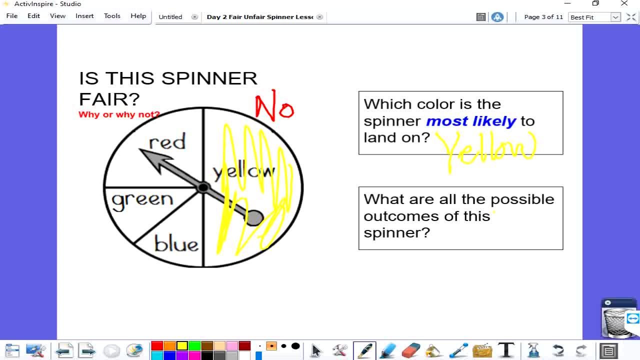 What are all the possible outcomes of this spinner? What does that mean? That means is: if I were to spin the spinner, what are all the possible Colors I could land on? Well, I know I can land on yellow. I can also land on red. 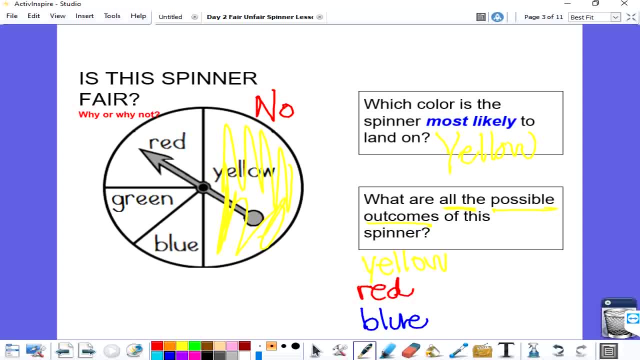 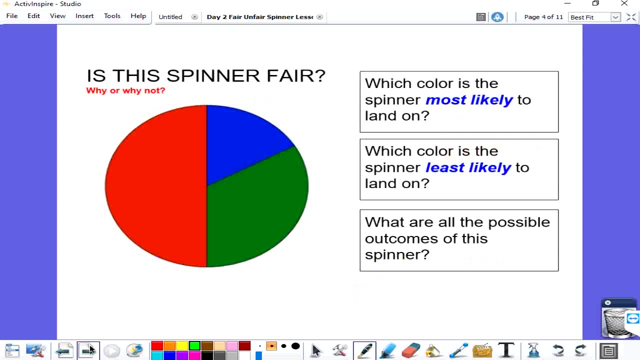 I can also land on blue And I can also land on green. So there are four possible outcomes if I were to spin that spinner. Let's take a look at another spinner. Is this spinner fair? Why, or why not? Well, looking at this spinner, I know it's not fair because there are three colors. 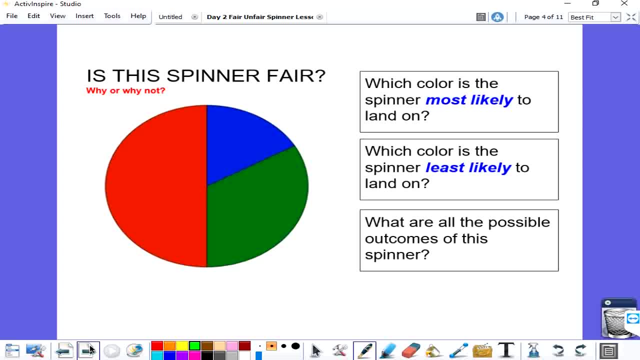 And each of those colors do not have the same size pieces, so it's not going to be fair. So my answer would be no. Which color is the spinner most likely to land on? Well, looking at the spinner, red has the biggest piece of that spinner, so I know it's most likely to land on red. 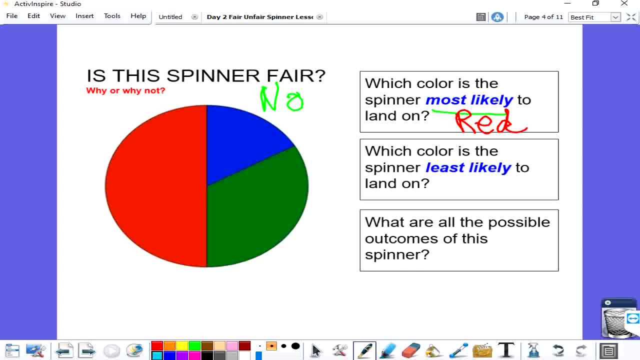 Which color is the spinner least likely to land on? Least likely means it probably will not happen. so I know that blue is the smallest piece. so I know that blue is least likely to land on. And finally, what are all the possible outcomes of that spinner? 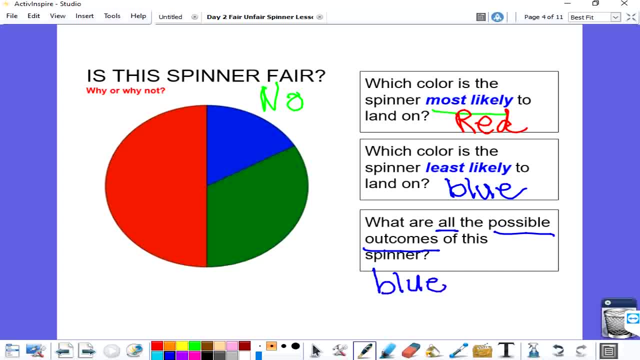 Well, I know, if I were to spin that spinner, I can spin a blue, I could spin a red or I can spin a green. So there are three possible outcomes for that. So I know, if I were to spin that spinner, I could spin a blue, I could spin a red or I could spin a green. 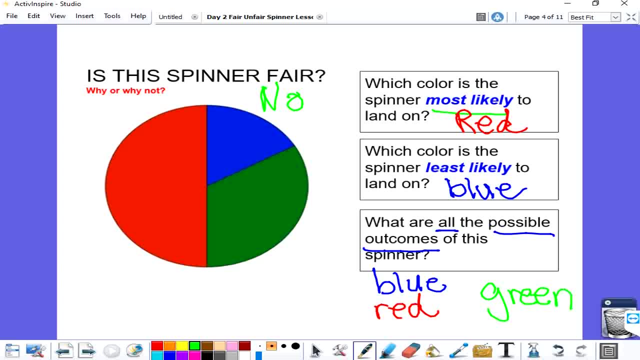 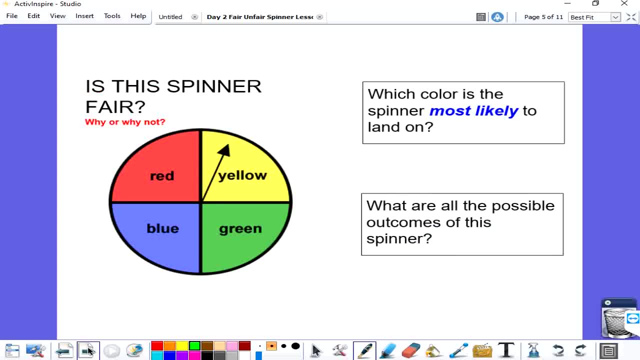 So there are three possible outcomes for that spinner. Okay, I'm going to take a look at another spinner. Is this spinner fair? Why or why not? Well, I noticed that all of the pieces are the same size, which is great. 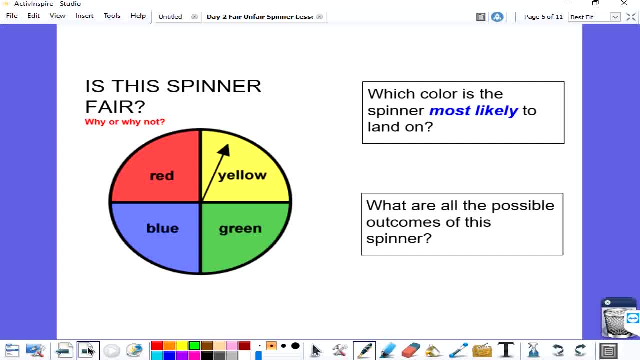 And each color has one piece. So I know that this spinner is fair. Yes, Yes, It is fair. So, looking at it, which color is the spinner most likely to land on? Well, I can't decide on that, because all of them have the same amount of space in that spinner. 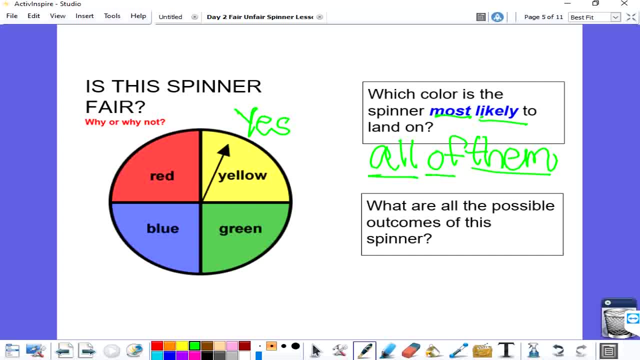 So it would be, all of them are equally likely or most likely to land on. And what are all the possible outcomes of the spinner? Well, I know, if I spun that spinner I could land on. I can land on a green, I can land on a red, I can land on a blue, or I can land on a yellow. 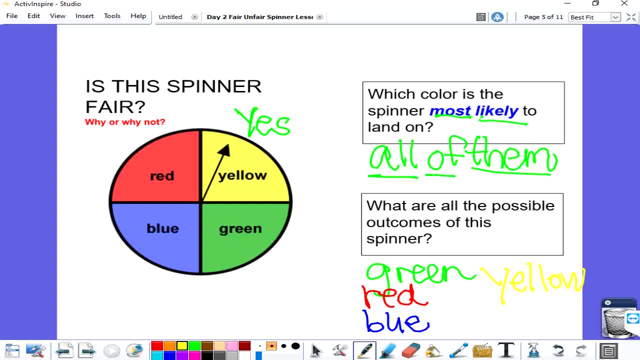 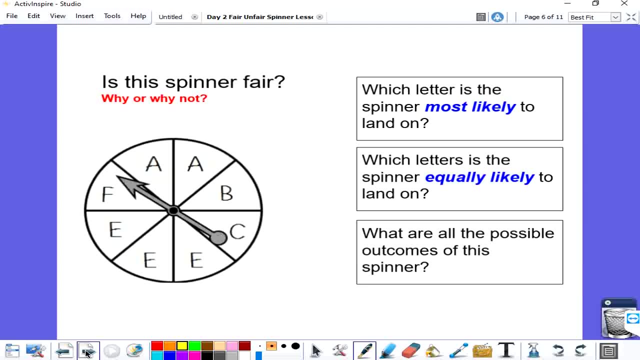 So there are four possible outcomes for that spinner. Now let's step it up a notch and take a look at this spinner. Do you think this spinner is fair? Why or why not? Yes, Well, let's take a look at that spinner. 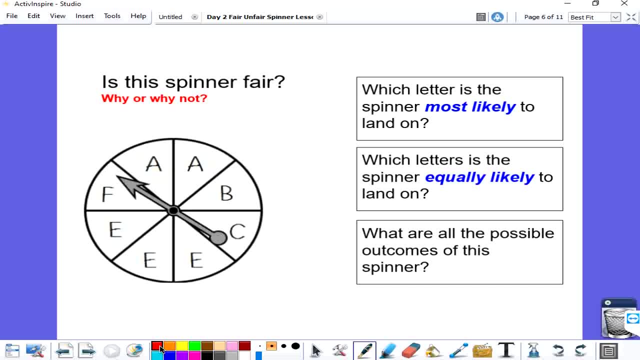 I know that. I know that there's eight pieces in that spinner and each piece is the same size. However, the letters do not have the same number of pieces, So let's take a look at the letters closely. A- there are two pieces with that letter. 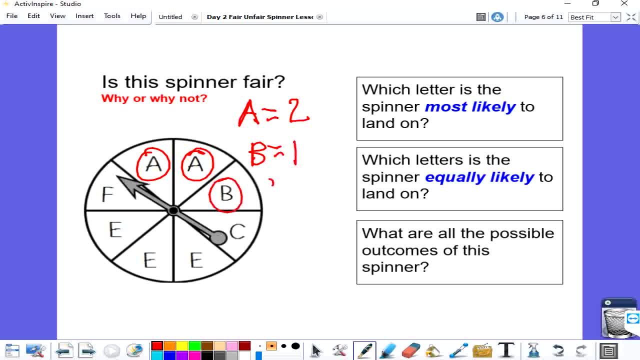 B has one piece, C has one piece, E, F has three pieces And F has one piece. So even though each of the size of the pieces on this spinner are the same size, the letters don't all have the same number of pieces, so it is not a fair spinner. 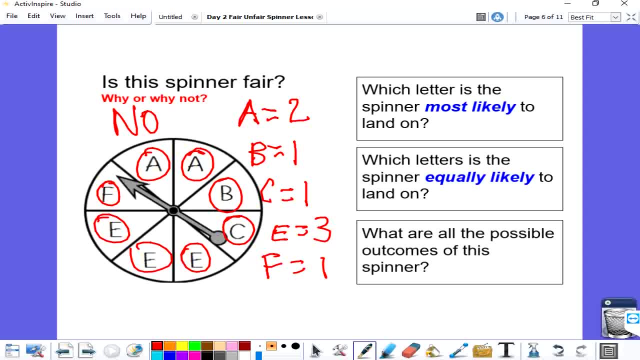 So, taking a look at that spinner, let's think Which letter is the spinner most likely to land on. Well, looking at the spinner, E has more spaces than any other letter, So E would most likely be the letter to land on. 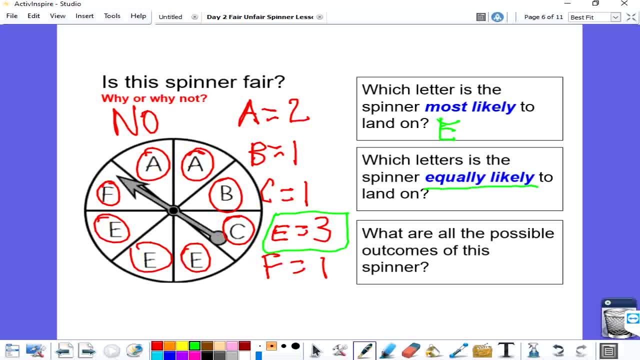 And then which letters is the spinner equally likely or have the same amount of probability to land on? Well, I can see that B, C and F all have the same number of pieces, So B, C and F all have an equally likely chance of landing on each letter. 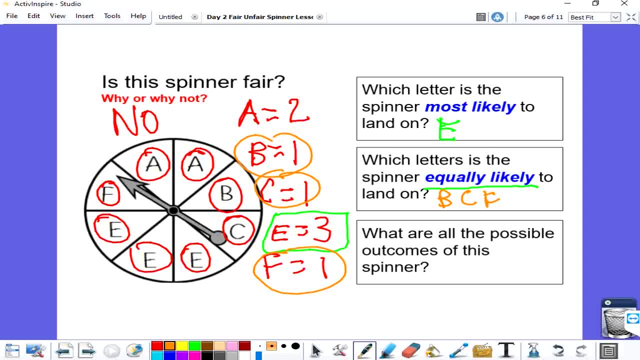 Well, I can see that B, C and F all have the same number of pieces, So B, C and F all have an equally likely chance of landing on each letter, of landing on that. What are all the possible outcomes of this spinner? Which means that 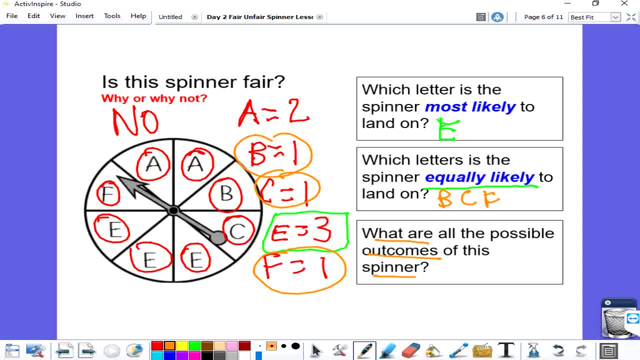 what are all the letters that you could possibly land on? Well, there is an, A, B, C, E and F, So there are five possible outcomes for this spinner. Now that we have a good idea of fair and unfair spinners and our probability statements, 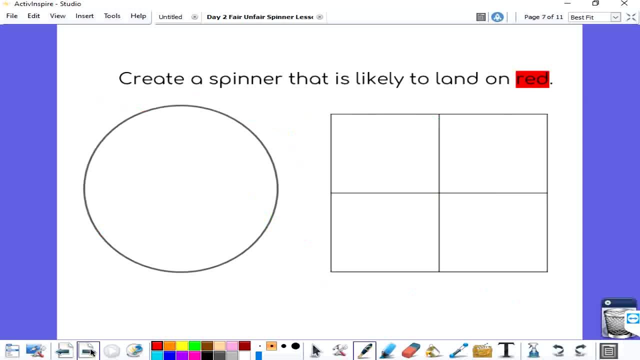 let's go ahead, and we're going to step it up a notch even further by creating spinners. We're going to create a spinner that is likely to land on red. Go ahead and pause this video and think about what that word likely means, Now that you've unpaused the video. 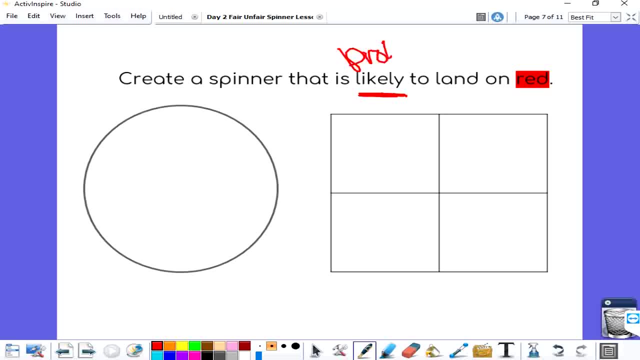 let's go ahead and create a spinner that is likely to land on red. Likely is that it probably will happen. Okay, so I want to make sure that red has more space on this spinner than any other color, So I can divide this spinner up into as many pieces as I want, as long as red takes up the 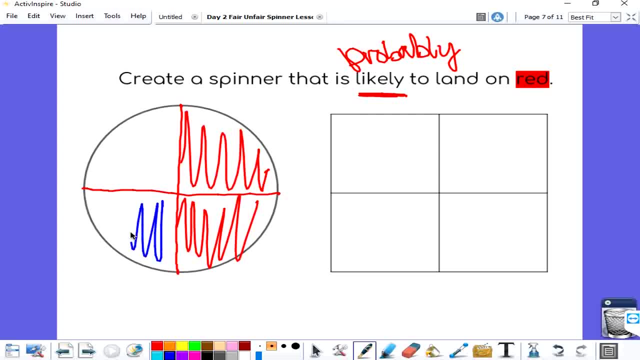 most amount of space on this spinner. So, as you can see that red has more space than any other color, Doesn't matter what other colors I use, as long as red takes up the most amount of space And I can fill in this square spinner just like my other spinner, Remember. 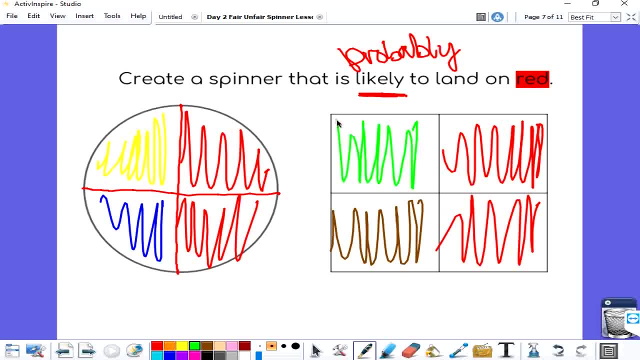 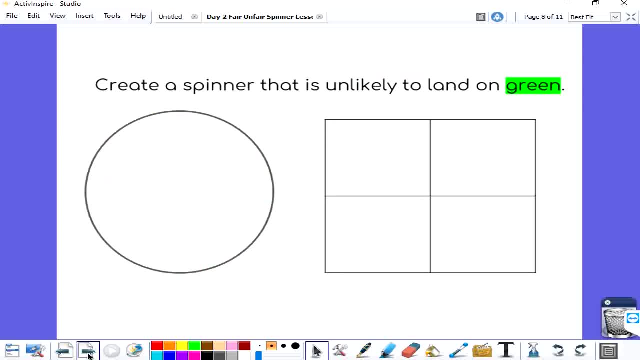 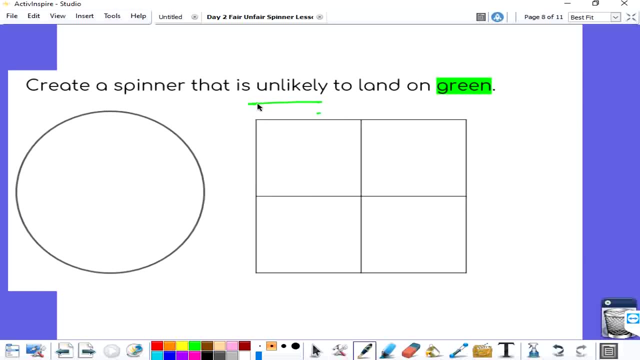 the other colors do not matter, as long as red has the most amount of space. because it is likely, Okay, let's create another spinner. It's asking us to create a spinner that is unlikely, Okay, unlikely small chance of landing on green. So we can only have a little space for. 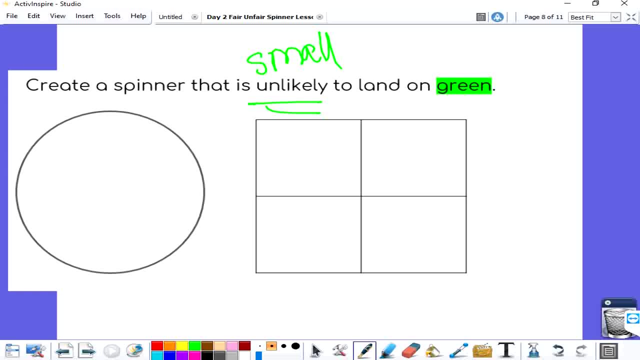 green, Everything else needs to be another color. So if I were just maybe put this spinner into six pieces- doesn't matter how many pieces, remember, as long as green has the smallest amount of pieces. I need to make sure that I have the smallest amount of pieces. 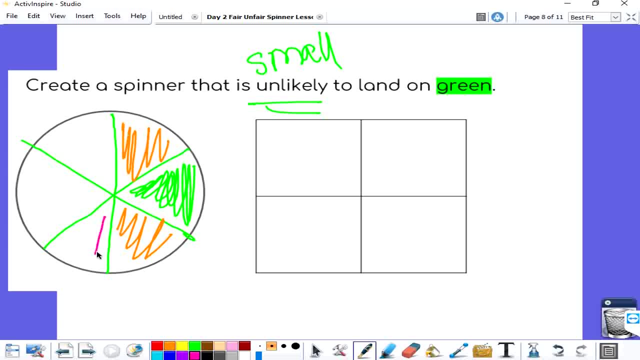 I need to make sure all of the other colors have more pieces than green. Okay, there's only one green piece on this spinner and the rest- orange- has more than green and pink has more than green, So I think we're good on that one. Let's take a look at our.